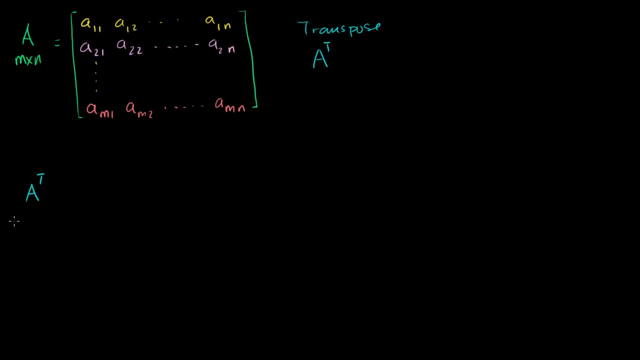 So my matrix A transpose is going to be a n by m matrix. Notice, I said m rows and n columns. Now this is going to have n rows and m columns. So what is this guy going to look like? What is he going to look like? 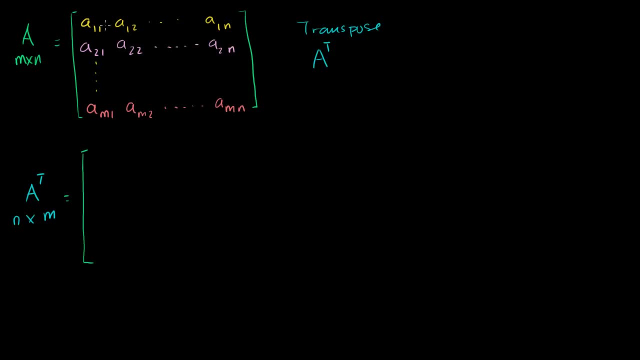 Well, I'm going to swap my rows and my columns, So my first row becomes my first column, So I'm going to have a 1, 1.. That entry is still going to be in that position, But now this entry is now going to be right here. 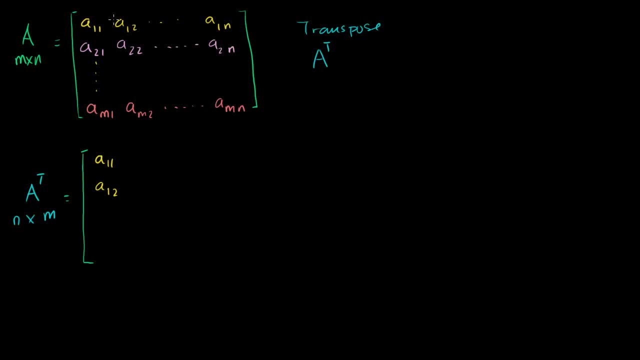 A 1, 2.. In my second row I have what I used to have in my second row, first column. I'm now going to have what I had in my second column, first row. I'm just going to go down all the way to A 1, n. 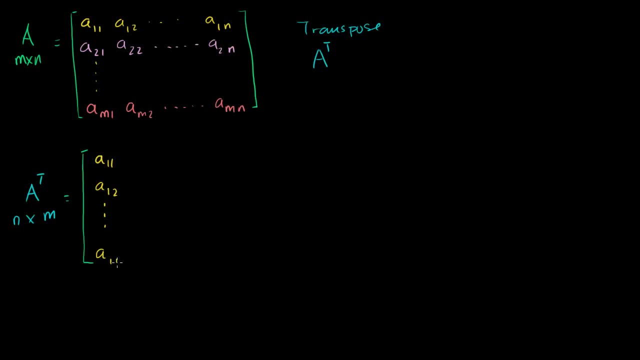 And that makes sense because I now have n columns. I'm sorry, I now have n rows. I had n columns before. Now I have n rows. Now this row. when I transpose it, it's going to look like this: A 2, 1, A 2, 2, all the way down to A 2, n. 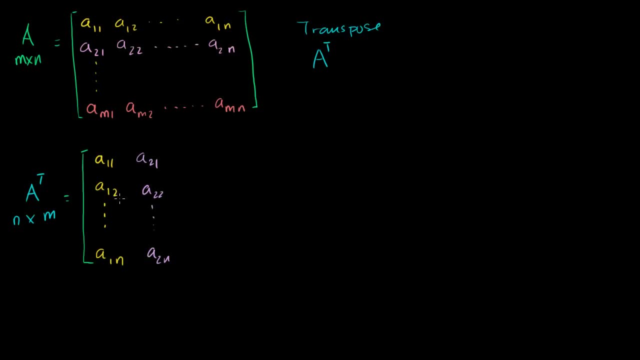 And it might be a little confusing for you right now to have this notation right there, because everything we've done so far, we've always said: hey, this first number is the row and the second number is the column. That's what we did up here. 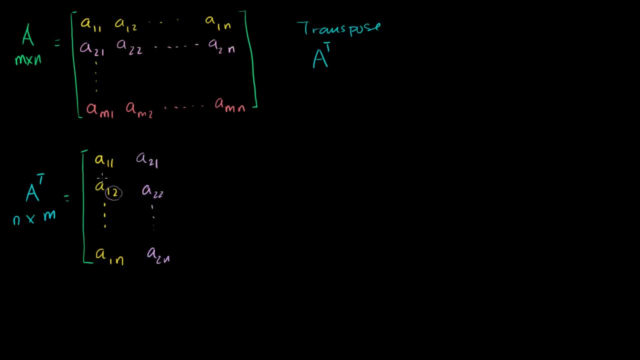 What I'm doing here. you can ignore that reference to the row, That reference to the rows and columns. you can just say: whatever we had here in my first row, second column, I now have here. So when you look at this, transpose, don't take these. 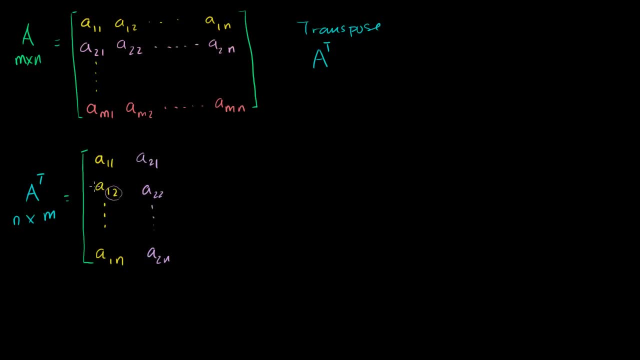 subscripts too literally, Or now you can kind of reverse your interpretation. This is now the first column, second row. This was the second row, first column, So I don't want you to get too confused with these subscripts. Just keep in mind we're taking all of the rows and 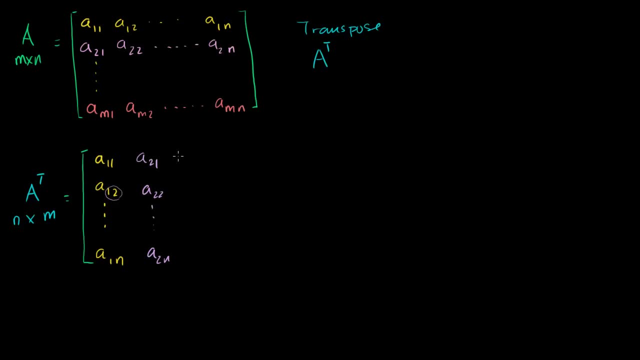 turning them into the columns to get the transpose, And then you just keep doing this And then this m-th row will now become the m-th column, a m 1, a m 2, all the way down to a m n. 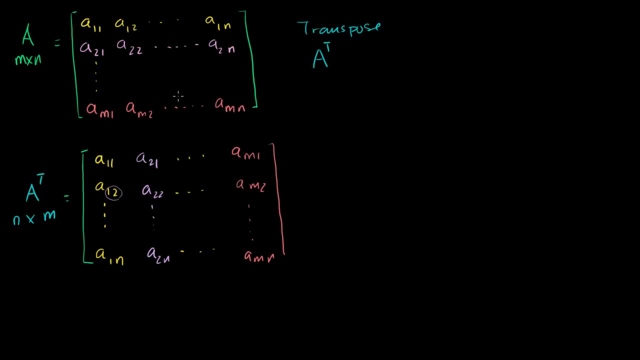 All the way down to a m? n. So this entry is now that entry. If you know, this entry is now that entry. That entry is now this entry. I think you get the idea. This is what a transpose is And sometimes, when you do it in the abstract, it can. 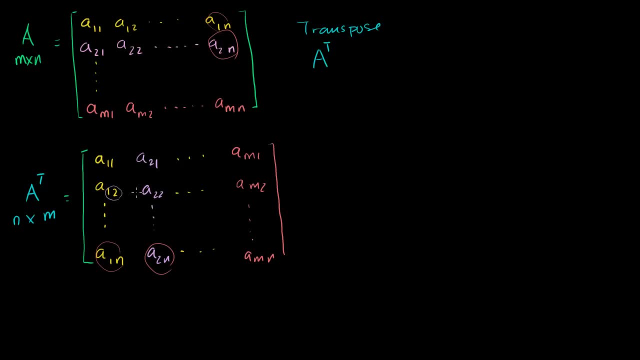 be a little confusing And we'll especially appreciate that once we do some of the proofs involving the transpose. But actually taking the transpose of an actual matrix with actual numbers shouldn't be too difficult. So let's start with the 2 by 2 case. 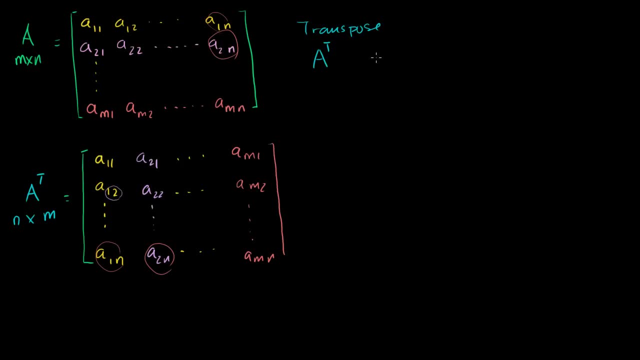 And I'll try to color code it as best as I can. So let's say I have the matrix. Let's say I define A. Let's do B. now We've already defined A. Let's say B is equal to the matrix. 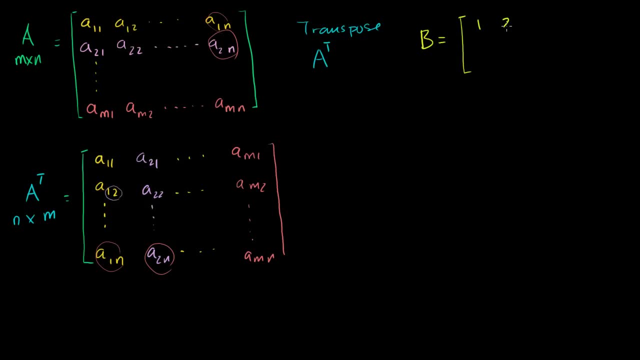 Let's say it's equal to the matrix 1,, 2,, 3, 4.. Those yellows are pretty close. But what is B transpose going to look like? B transpose is going to be equal to you. switch the rows. 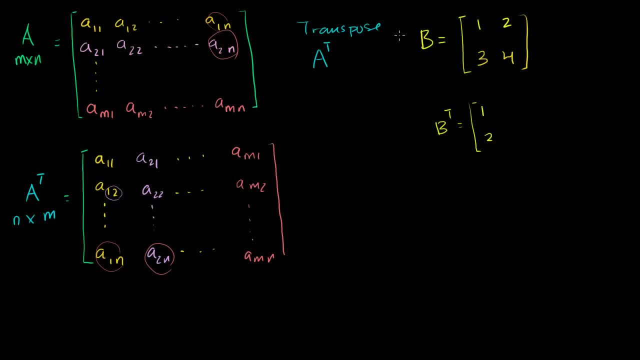 and the columns. so the first row will now become the first column 1,, 2, and the second row will now become the second column 3, 4.. Or you could do it the other way: The first column now became the first row and the second. 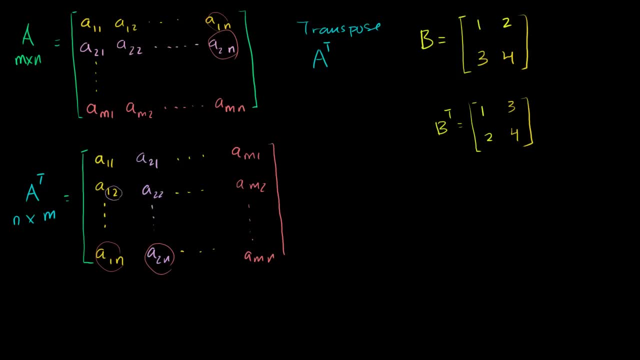 column now became the second row. Let's do an example. Instead of even doing a 3 by 3, let me do one that might be a little bit more challenging. I think this will make things clear. So let's say: I have the matrix C right here. 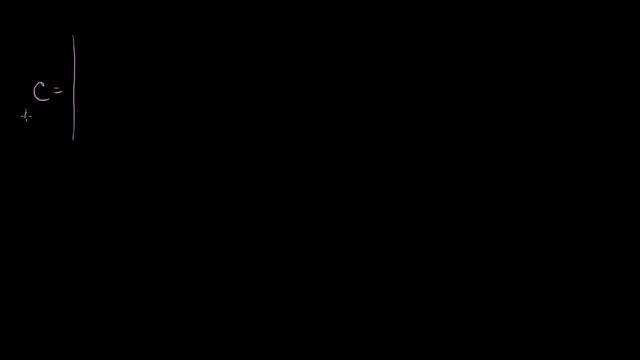 And let me make it a pretty big matrix. Let's say it is a 4 by 3 matrix right here. So let me just throw some numbers in there: 1. 0.. 0. Minus 1. 2.. 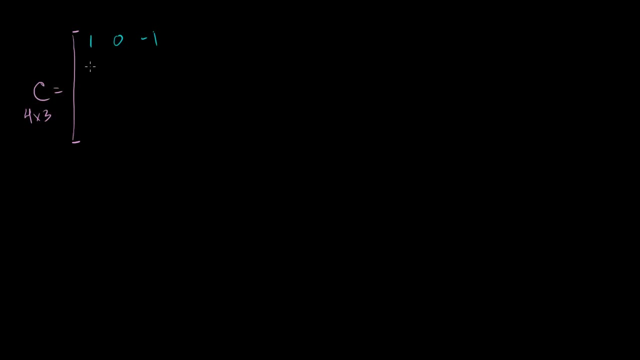 7.. Oh, I want to do it in different colors. Let me do that in a different color. So then I get 2, 7, minus 5.. Then I get 4, minus 3, 2.. And I have to do one more row here. 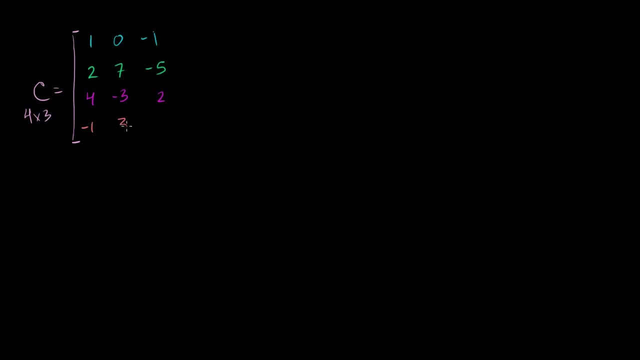 So let me just make that minus 1,, 3, and 0.. That is my matrix C. So what is? let me do that in. I like to BST. It would be aesthetically pleasing, So let me close the bracket in the same color. 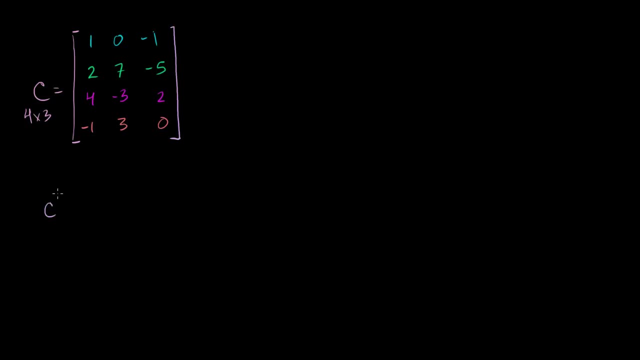 So what is C transpose going to be? So C transpose, let me do that in a different color. C transpose is now going to be a 3 by 4 matrix And essentially it's going to be the matrix C, with all the rows swapped for the columns. 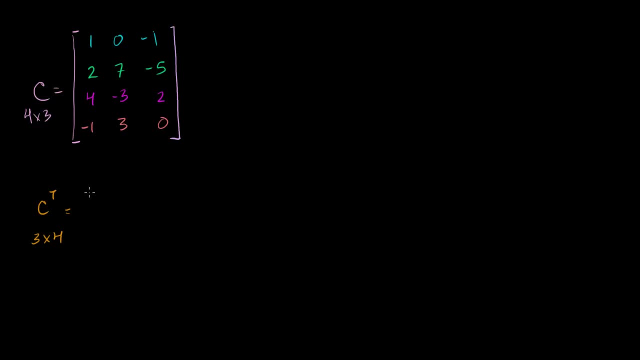 or all the columns swapped for the rows. So it's now going to be a 3 by 4 matrix And that first row There is now going to become the first column: 1, 0, minus 1.. The second row here is now going to become the second column. 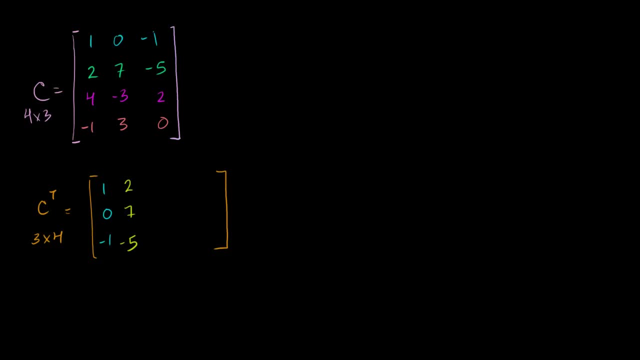 2, 7, minus 5.. I didn't use the exact same green, but you get the idea. This third row will become the third column: 4, minus 3, 2.. And then, finally, the fourth row will become the fourth column. 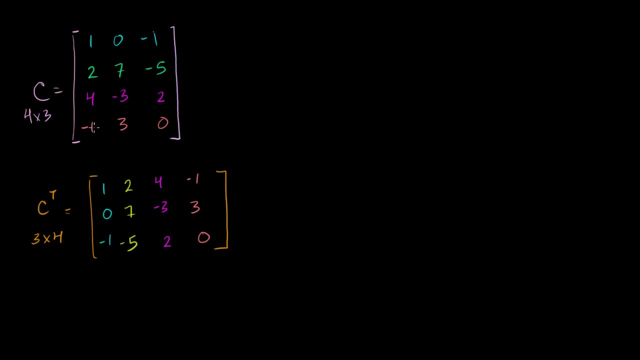 minus 1,, 3, and 0.. So all we did is, if this guy was, let's say, this guy was in the position, this guy was in the second row. second row. second row, third column. third column. 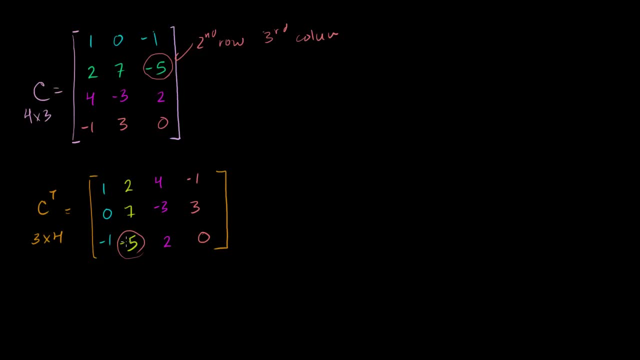 Now that same guy is in the what He is in the second column. second column and the third row, The third row. All we did is switch the rows and the columns. We could do it with another. Let's see. 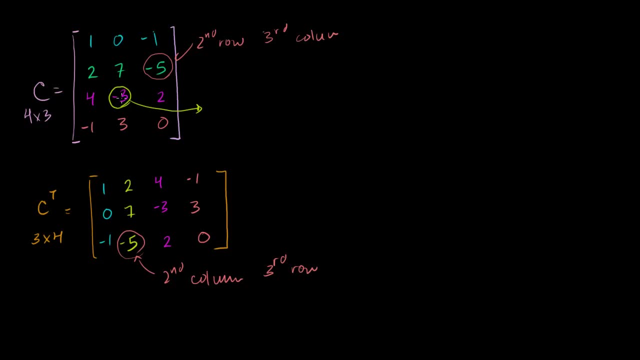 Let's do it with this one right here. This guy right here is in the third row, 1,, 2,, 3, and the second column, And when you go down here, this guy is now in the third column and the second row. 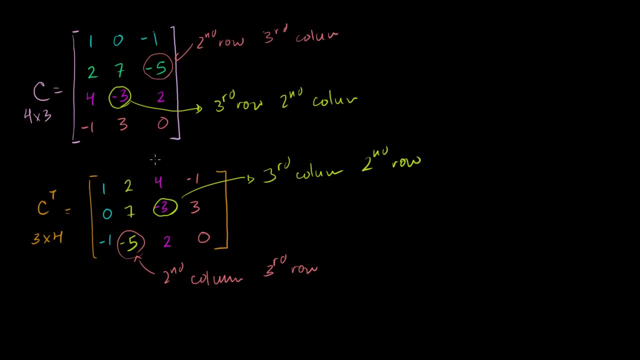 That's all a transpose is. And, just as a little interesting thing, what happens if we take the transpose of the transpose? So what happens if we take c transpose and then transpose that? What is that going to be? equal to Well to go from c to c transpose.